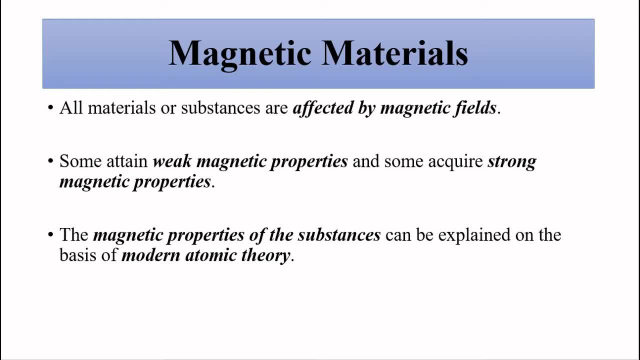 magnetic field. it gets affected. Now some they get weakly magnetized. that means they attain magnetic properties to a very small extent, while some acquire strong magnetic properties Magnetized to a large extent. Now why some get weakly magnetized, some get strongly magnetized. 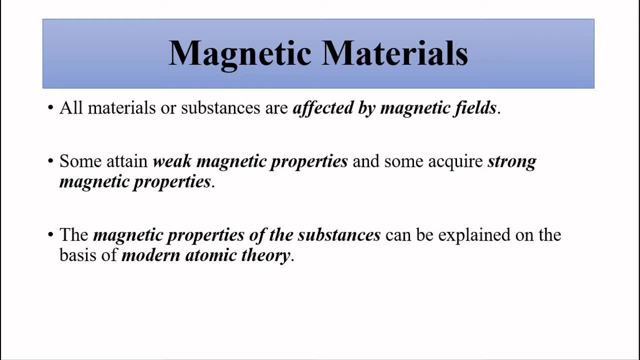 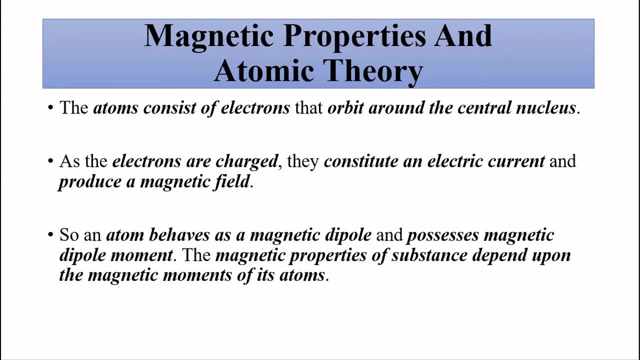 that can be expressed on the basis of the atomic theory. Now we have already discussed magnetic dipole, how atom behaves as a magnetic dipole. So we know that an atom it consists of two electrons orbiting around the nucleus, So the revolving electrons around the nucleus. 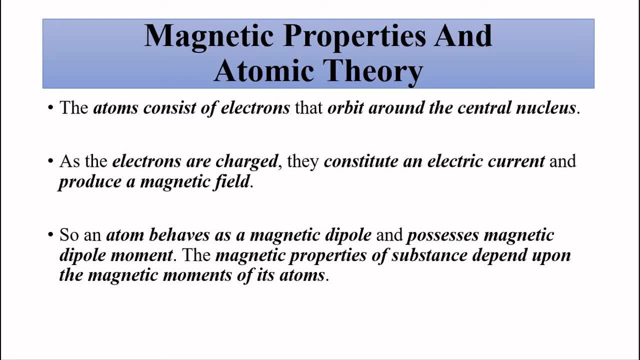 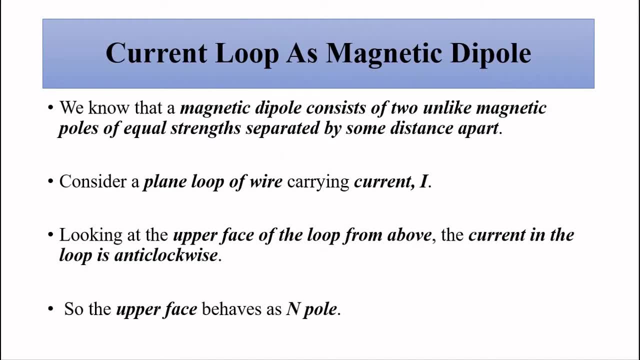 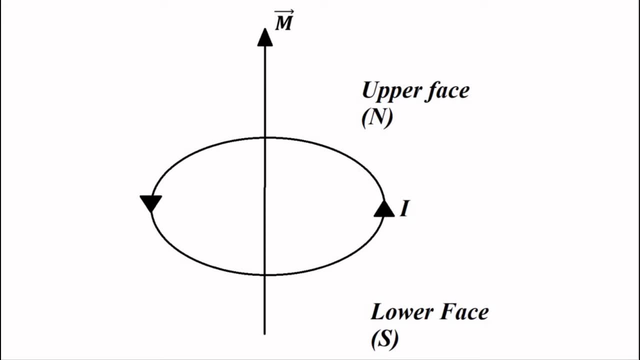 they behave as an electric current and produce a magnetic field. Now we have already discussed how a current loop it behaves as a magnetic dipole. So suppose we consider a plane loop of current carrying a current i When we see the top face from the top side, the current 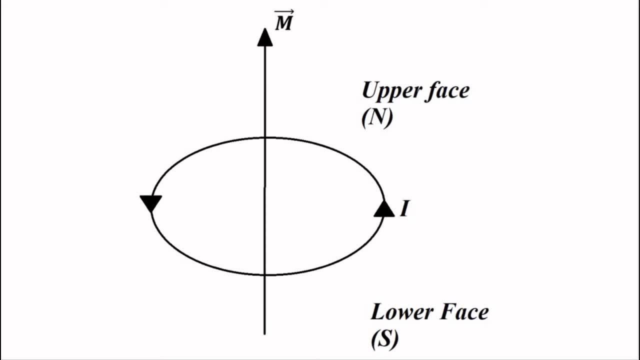 appears to be moving in anticlockwise direction. that is why it acquires north pole. When we look at from the bottom, it appears as if the current is moving in clockwise direction. that is why it acquires south pole. Similarly, when an electron, it revolves around the nucleus with a certain velocity. a current 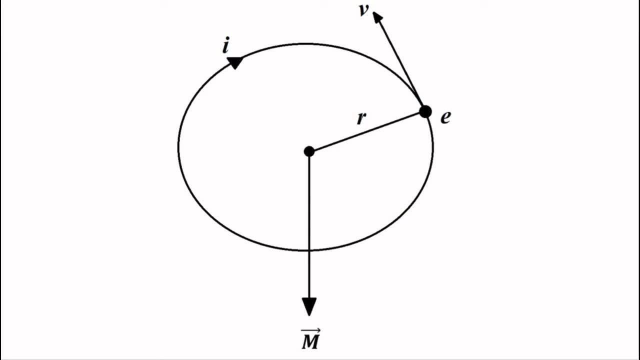 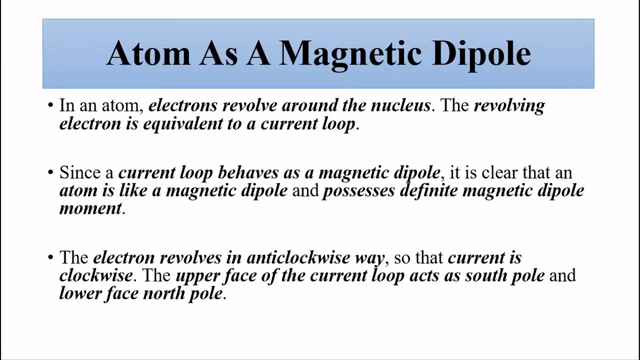 flows in the opposite direction, because current direction is always opposite to the electron movement electron movement direction. So this current flowing is similar to this, you know, plane loop of current and that is why the atom, it behaves as a magnetic dipole as a whole, because of the movement of electrons. 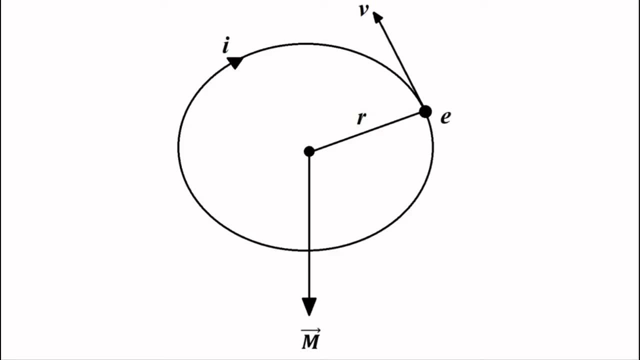 in the various orbits around the nucleus. So this magnetic behavior of atom, it is expressed as the orbital magnetic movement which is given by n, e, h, by 4 pi m, where n is the number of orbit, e is the electronic charge, h is 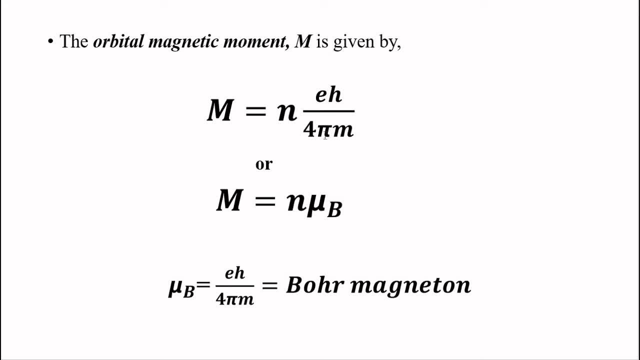 Planck's constant m is the mass of the electron. Here this e h by 4 pi m is called as Bohr magneton. ok, So this is. This is why the materials they behave, you know they respond to a magnetic field, or they. 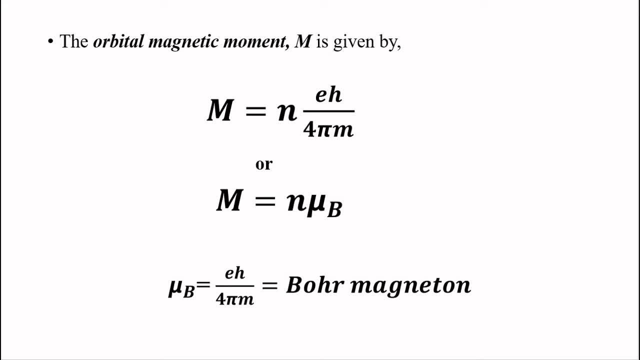 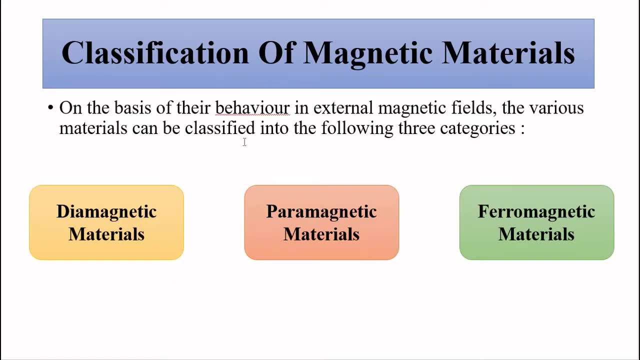 acquire magnetic properties. So, on the basis of this, magnetic materials can be classified into three categories: Diamagnetic materials, paramagnetic materials, ferromagnetic materials. In this video, we will be discussing only about diamagnetic materials, paramagnetic and ferromagnetic. 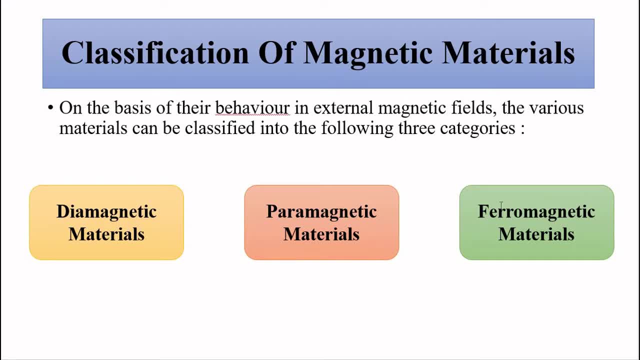 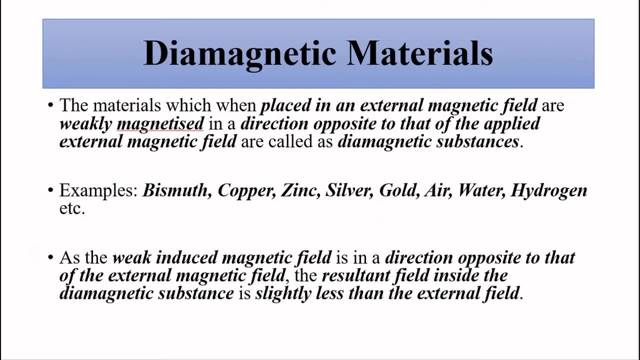 materials. Diamagnetic materials we will be discussing in separate videos. So diamagnetic materials. So diamagnetic materials are those when placed in an external magnetic field they get weakly magnetized or they acquire magnetic properties to a small extent in the opposite direction. 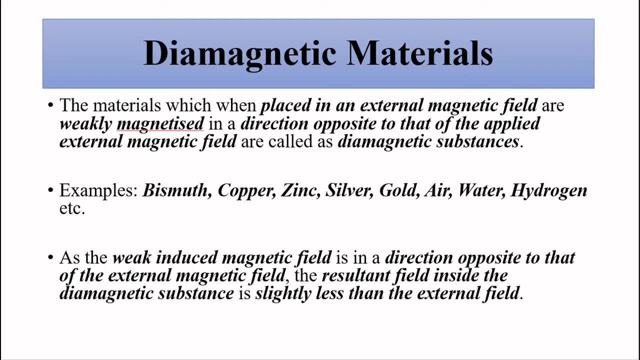 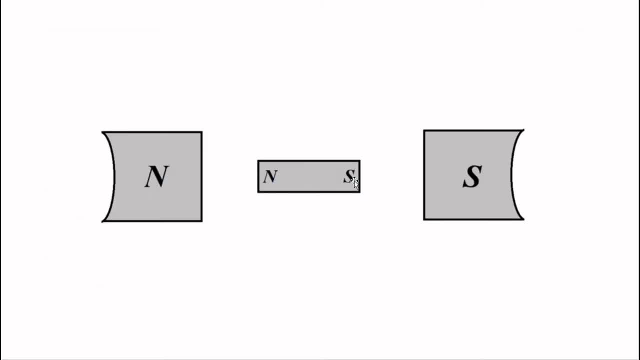 to the applied external field. So it means that when This diamagnetic material is placed in the external magnetic field produced by this permanent magnet, This extreme end which is facing the north pole of the permanent magnet, it acquires a north pole and the other extreme end facing the south pole of the permanent magnet, it 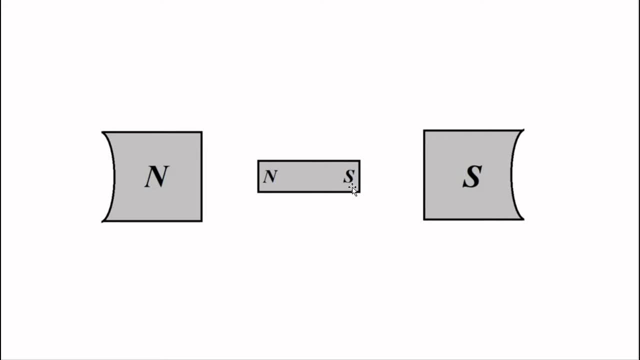 acquires a south pole. So that's why This End Repels This north pole and this south pole repels this south pole. So it always gets repelled because of the external magnetic field. This is what diamagnetic behavior is. 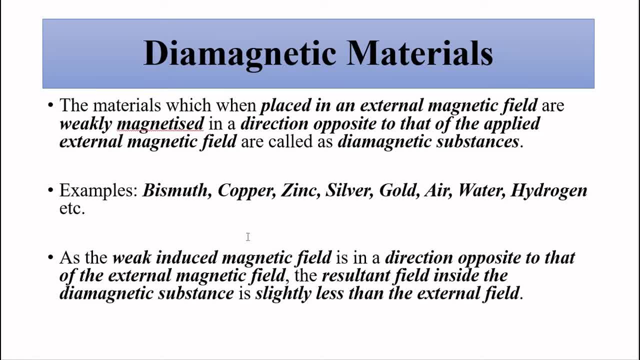 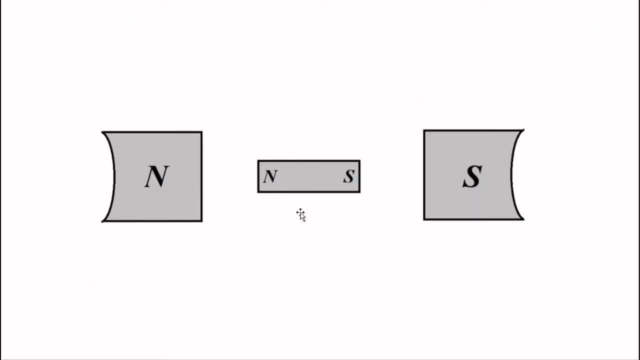 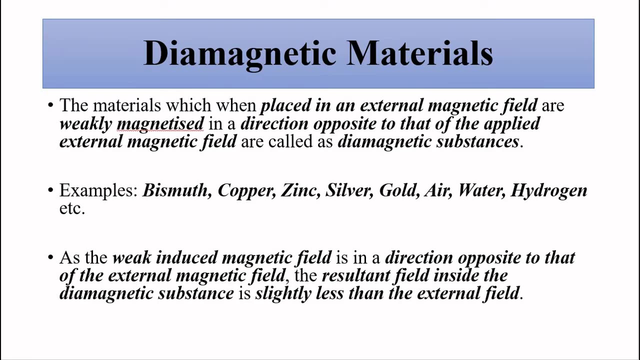 Examples of such materials are bismuth, copper, zinc, silver, gold, air, water, hydrogen, etc. So here The Resultant magnetic field inside the material is always less than the external field, which is evident because it is weakly magnetized, and it is. it is a very weak form of magnetism. 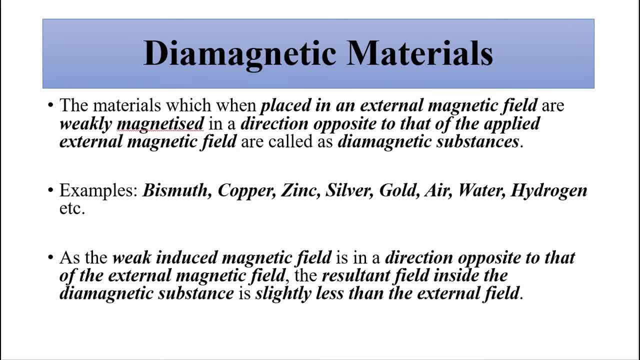 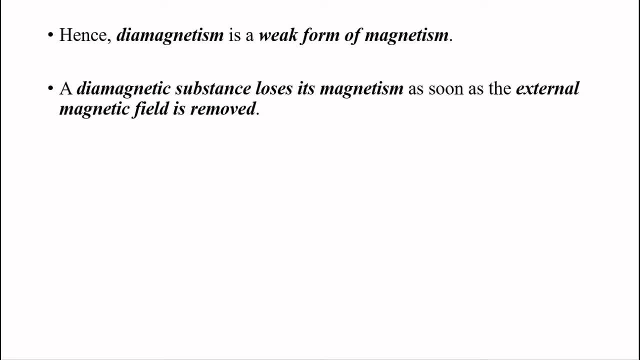 and as long as the external field is removed, the material, it loses its magnetic properties. Okay, So Why The Demagnetic Materials behave in that way? Why they acquire a weak form of magnetism, Why they are weakly magnetized. 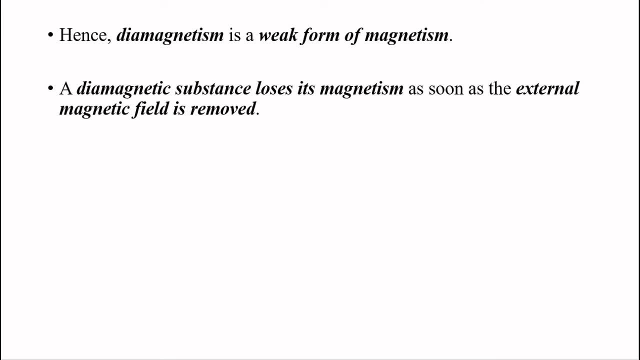 So again here the magnetic dipole moments come come into play. So again the electrons in the various orbits of the atom. they revolve around the nucleus and possess magnetic moments. in case of diamagnetic materials, What happens Is That The magnetic dipole moments 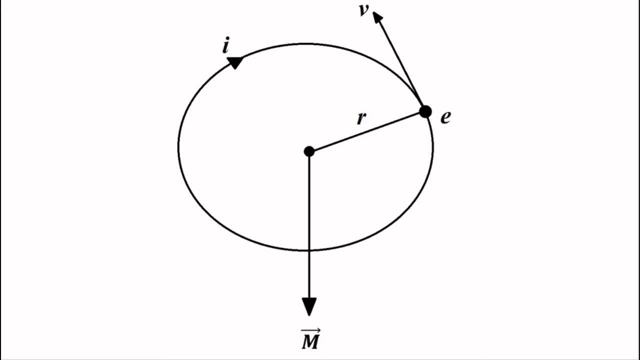 They Always exist in opposite Pairs. Okay So, as they exist in opposite pairs equal in magnitude, opposite in direction, So they always cancel each other out. Okay So, the magnetic dipole moments in diamagnetic materials. they exist in opposite pairs equal. 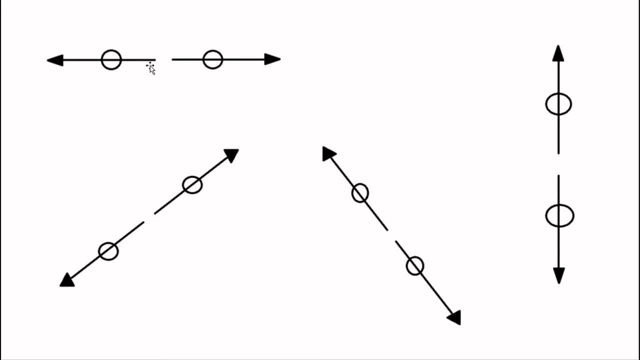 in magnitude opposite in direction, so they always cancel each other out. So the magnetic dipole moments in diamagnetic materials: they exist in opposite pairs equal in magnitude, opposite in direction, so they always cancel each other out. So the magnetic dipole moments in diamagnetic materials: they exist in opposite pairs equal 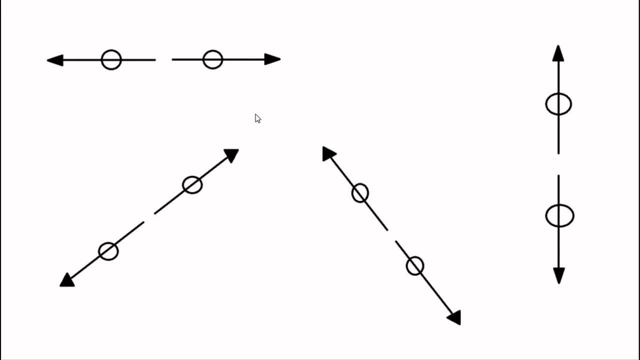 in magnitude opposite in direction, so they always cancel each other out. So the magnetic dipole moments in diamagnetic materials: they exist in opposite pairs equal in magnitude, opposite in direction, so they always cancel each other out. So the magnetic dipole moments in diamagnetic materials: they exist in opposite pairs equal 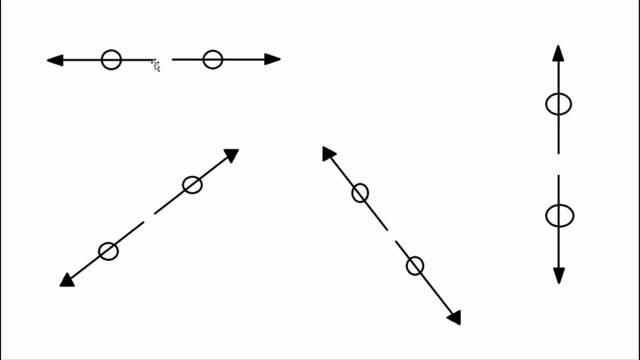 in magnitude opposite in direction, so they always cancel each other out. So the magnetic dipole moments in diamagnetic materials: they exist in opposite pairs equal in magnitude, opposite in direction, so they always cancel each other out. So the magnetic dipole moments in diamagnetic materials: they exist in opposite pairs equal 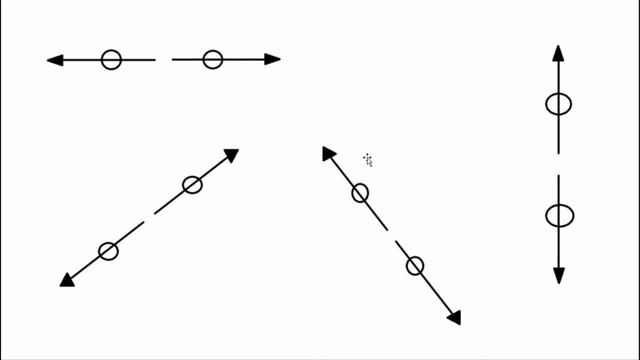 in magnitude opposite in direction, so they always cancel each other out. So the magnetic dipole moments in diamagnetic materials: they exist in opposite pairs equal in magnitude, opposite in direction, so they always cancel each other out. So the magnetic dipole moments in diamagnetic materials: they exist in opposite pairs equal 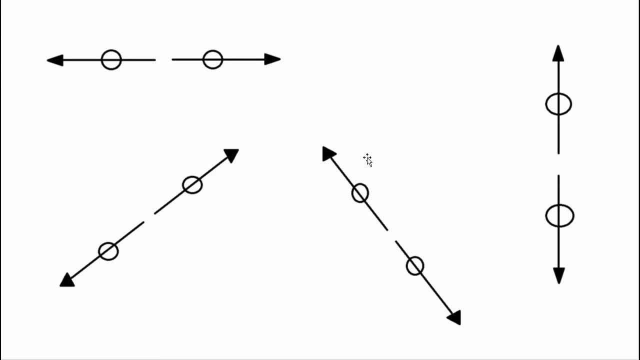 in magnitude opposite in direction, so they always cancel each other out. So the magnetic dipole moments in diamagnetic materials: they exist in opposite pairs equal in magnitude, opposite in direction, so they always cancel each other out. So the magnetic dipole moments in diamagnetic materials: they exist in opposite pairs equal 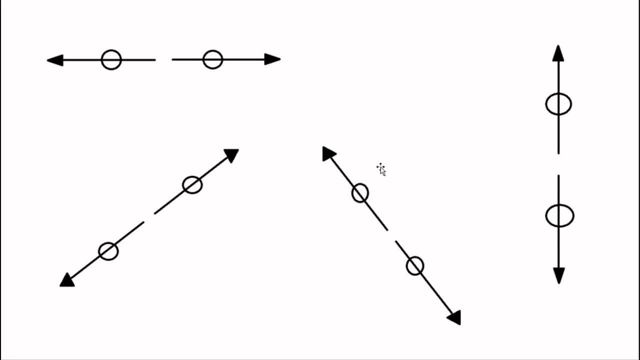 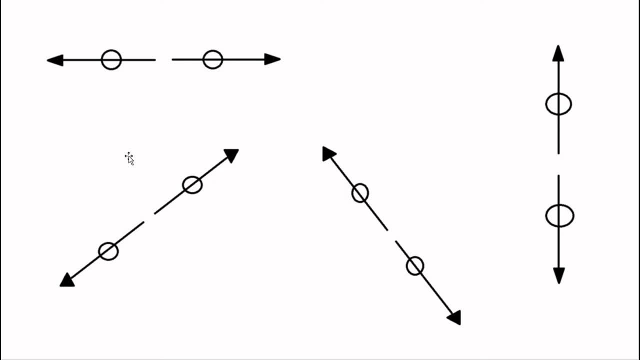 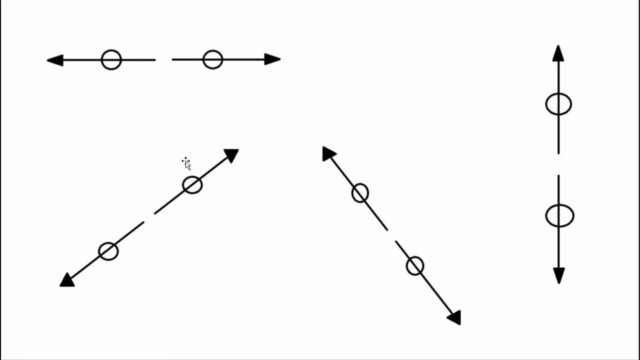 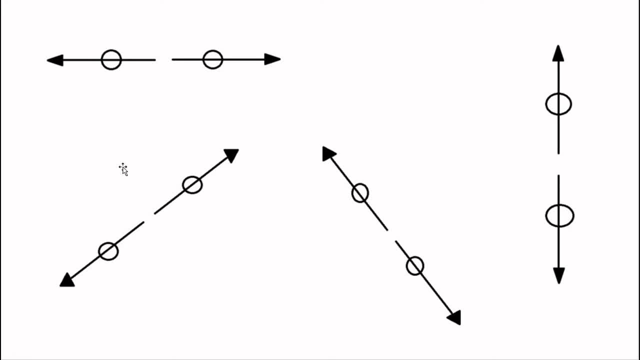 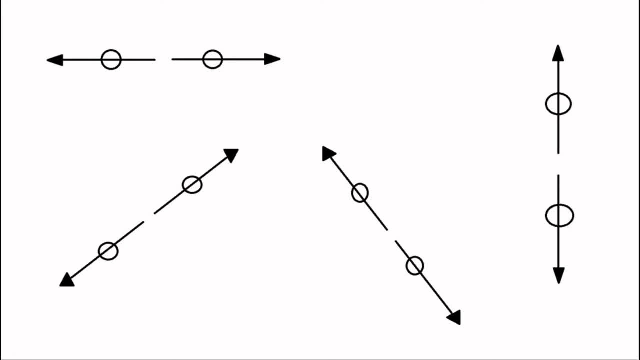 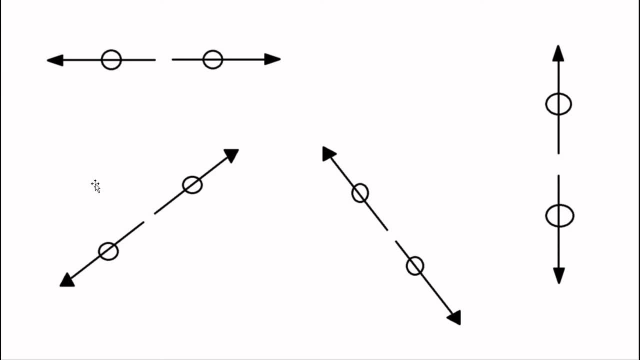 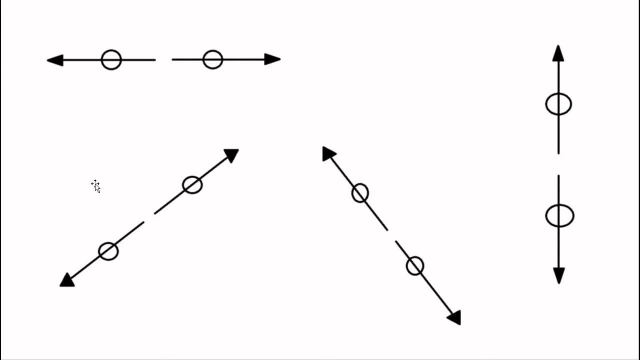 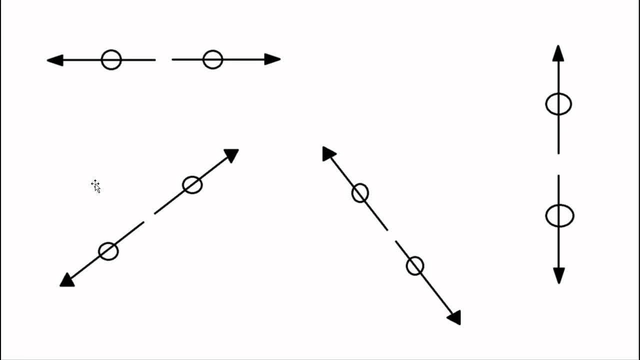 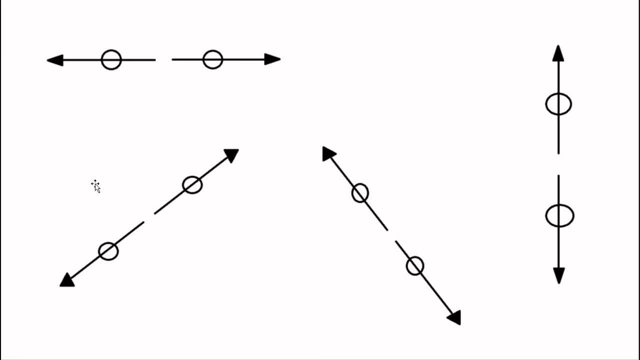 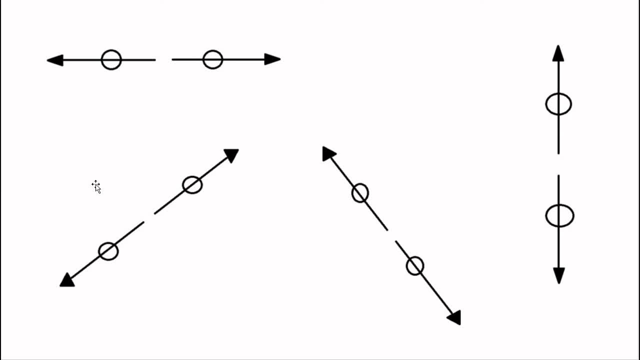 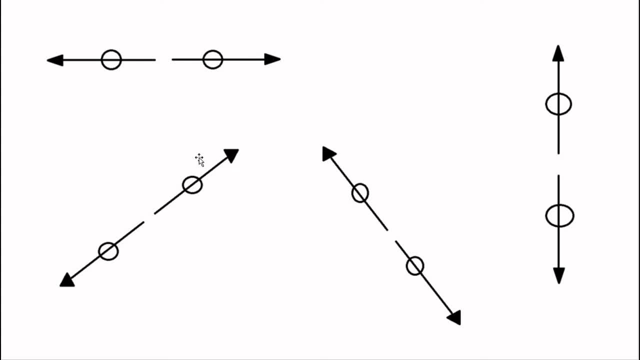 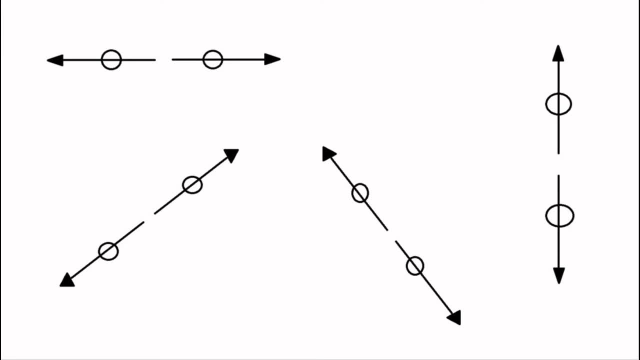 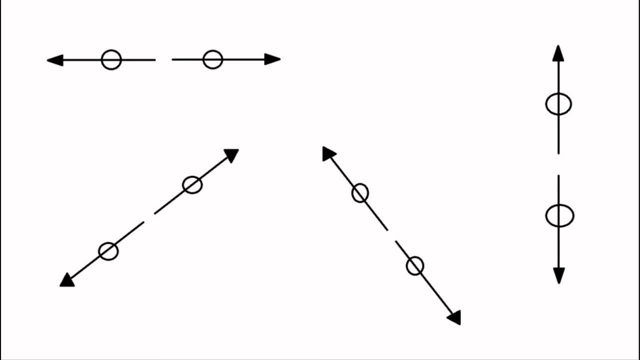 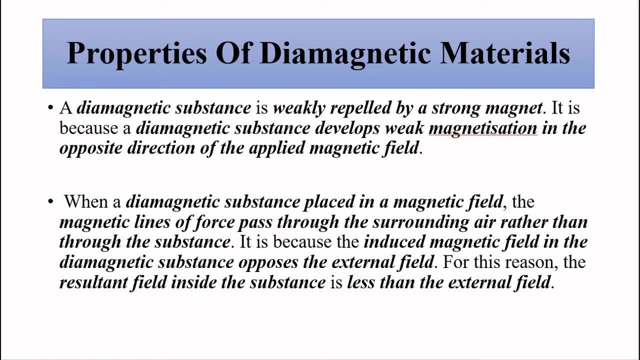 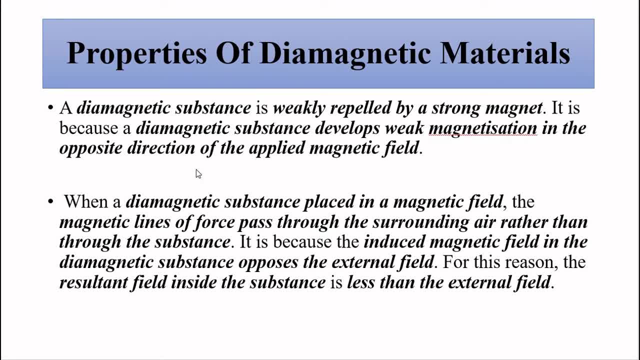 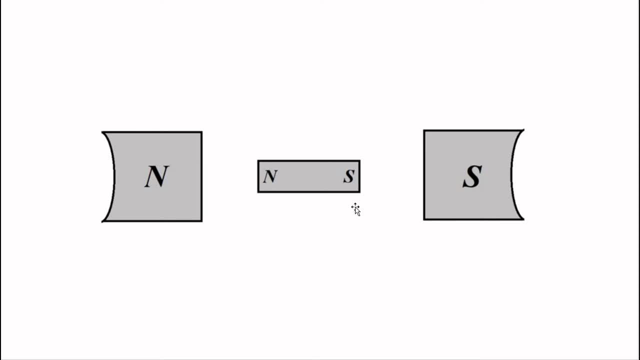 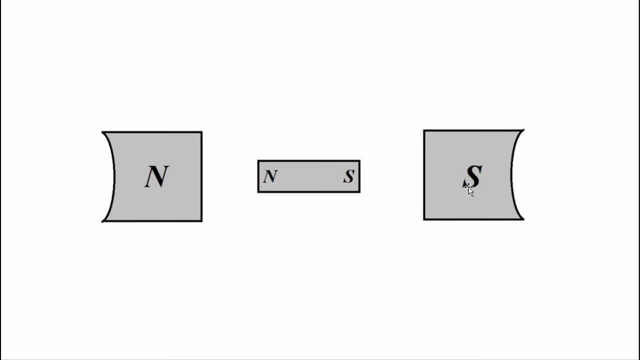 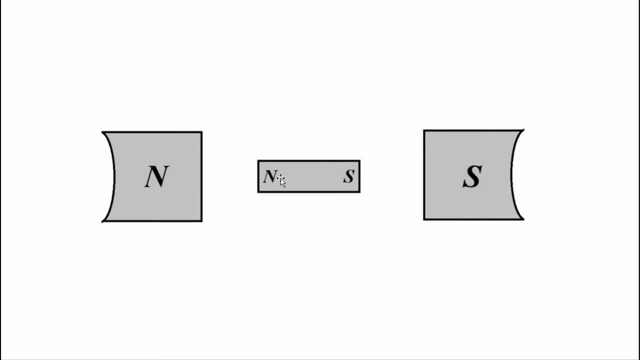 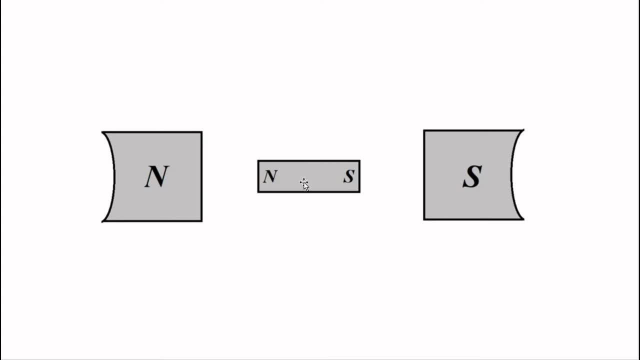 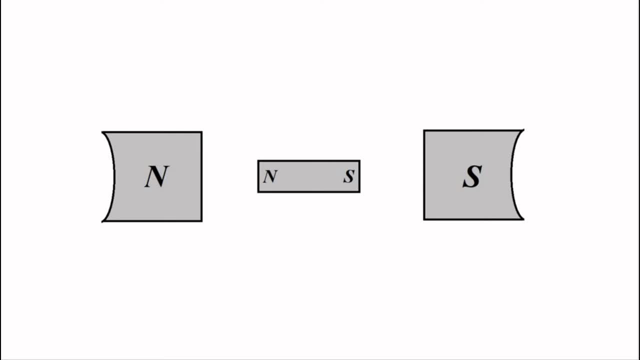 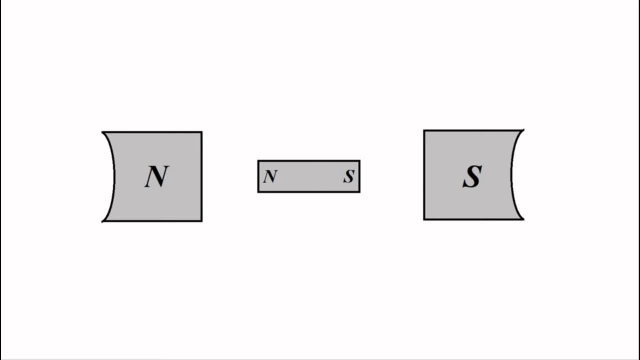 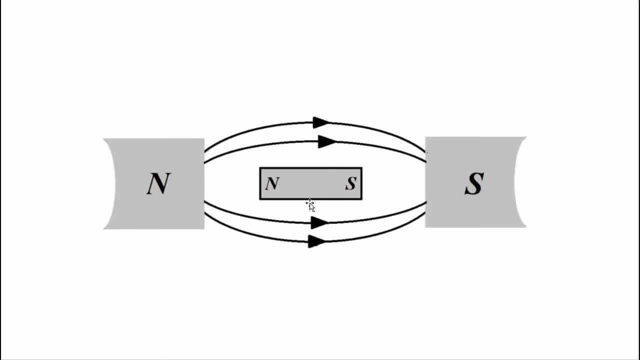 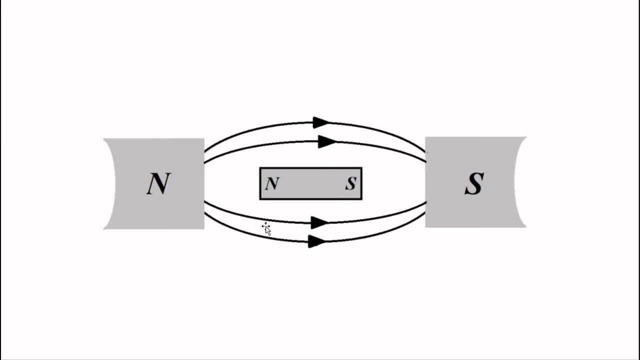 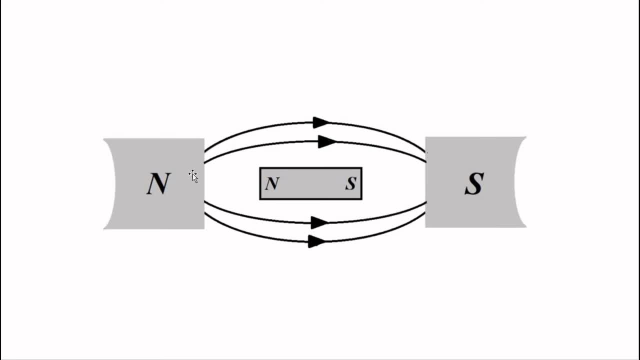 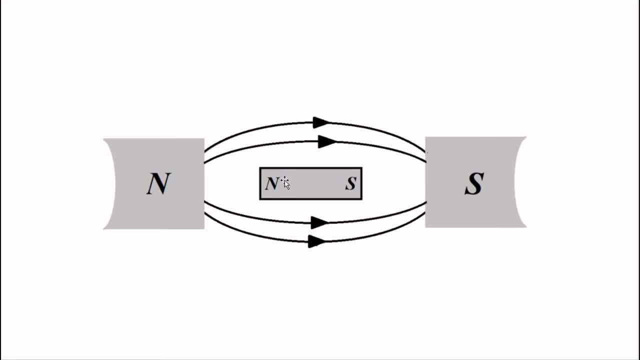 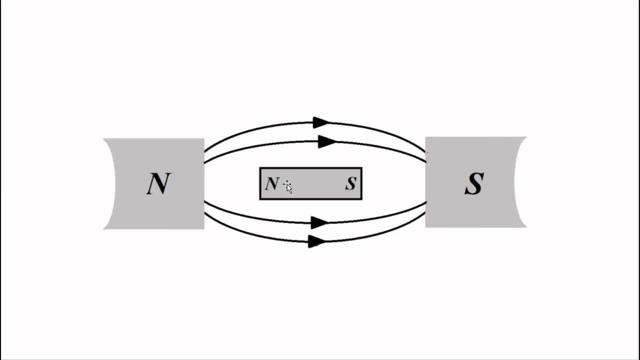 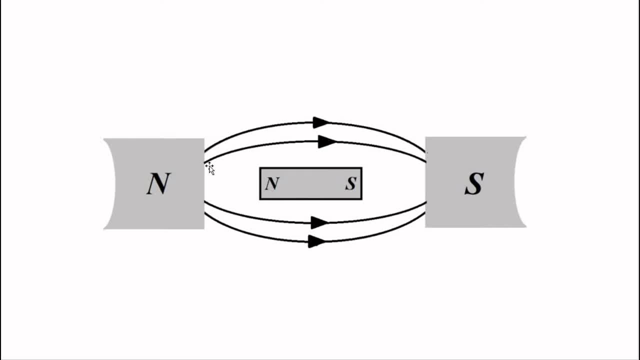 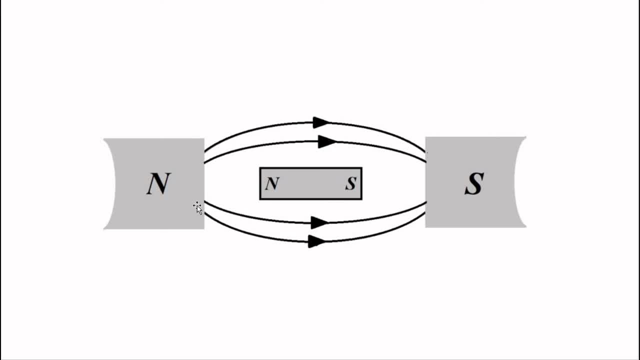 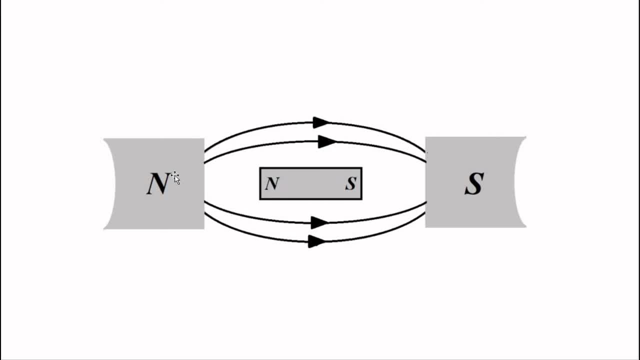 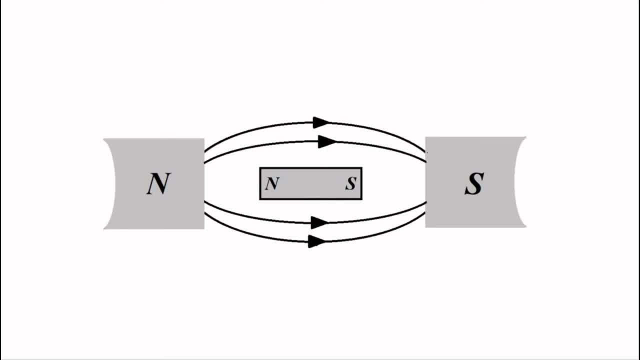 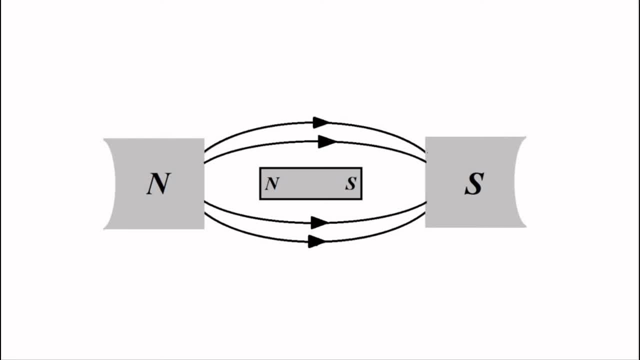 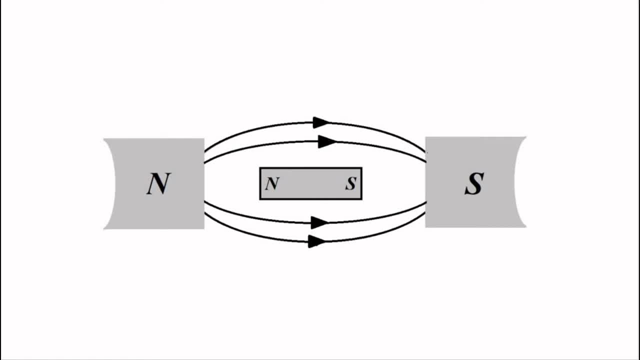 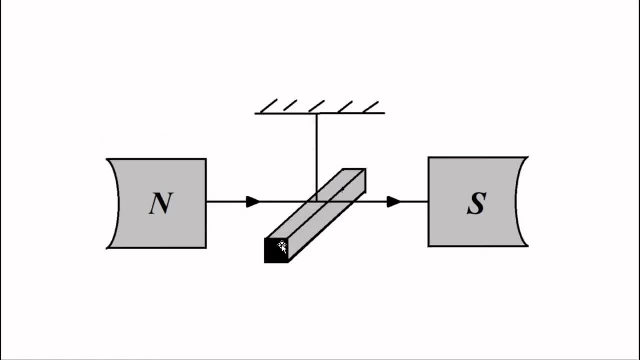 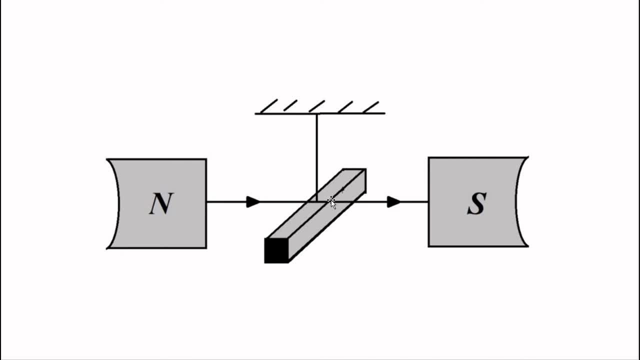 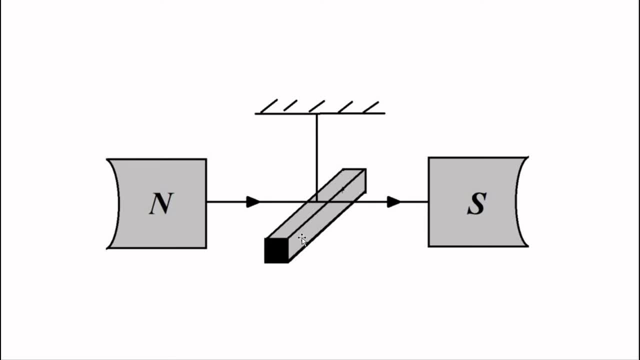 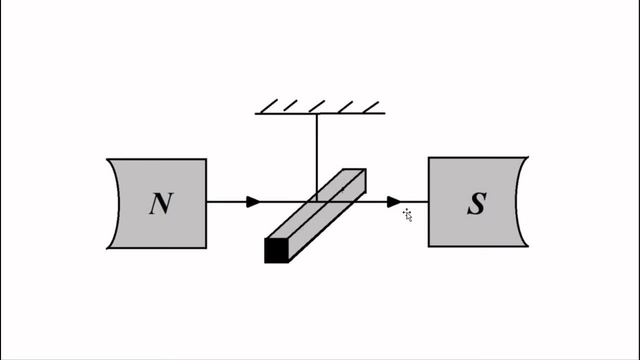 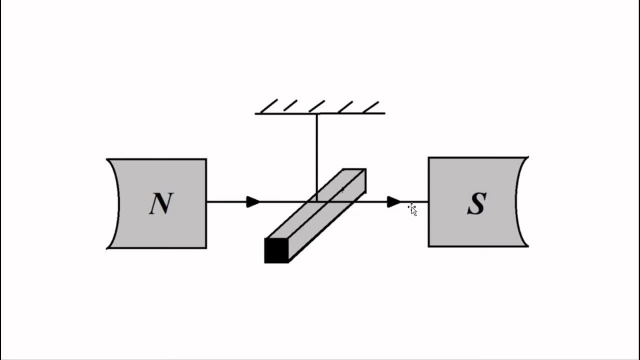 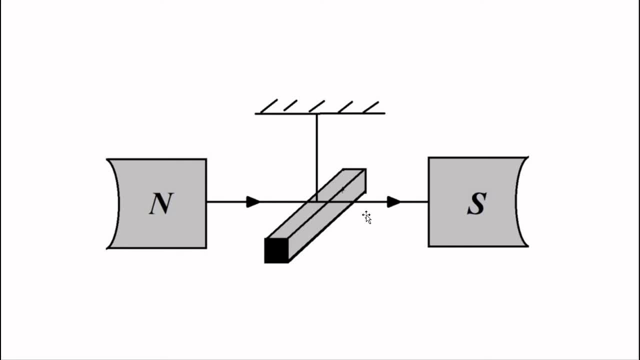 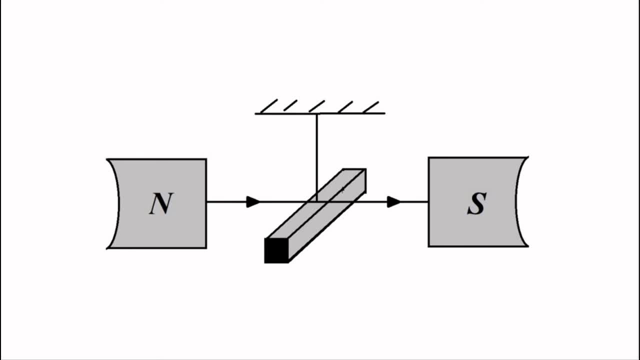 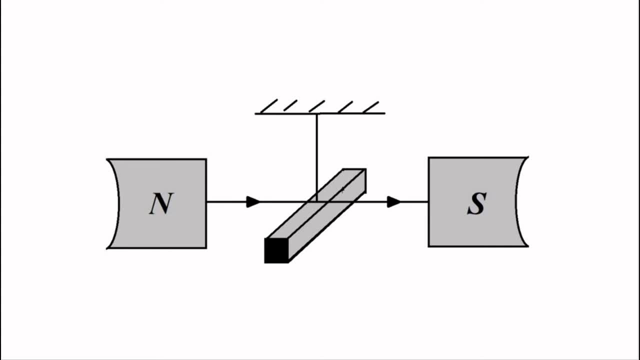 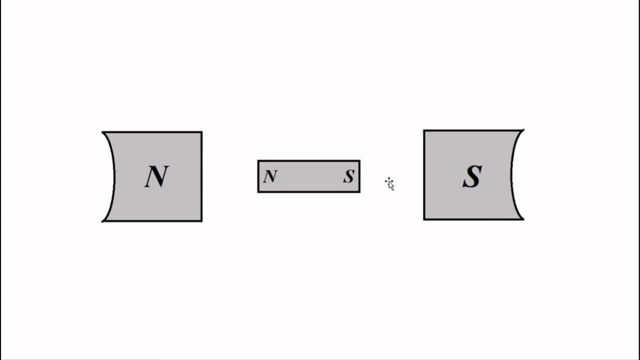 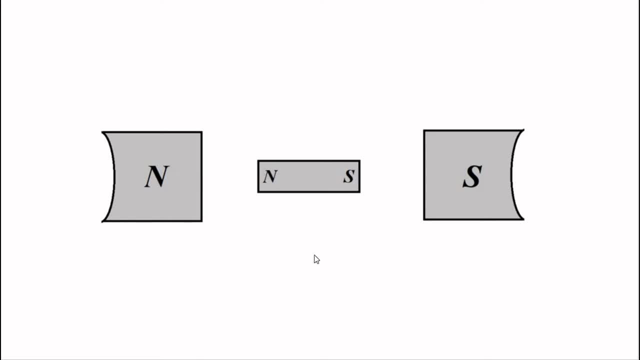 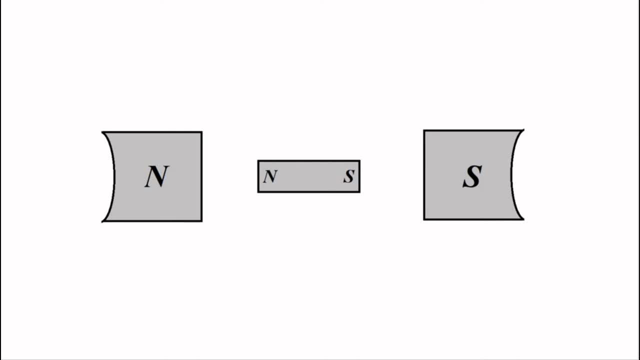 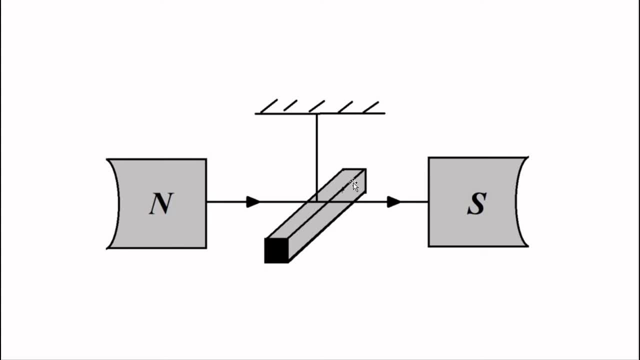 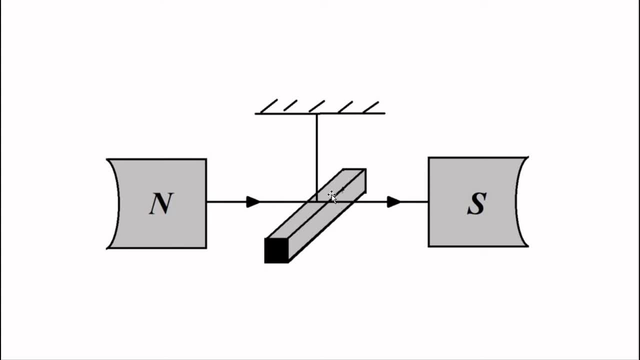 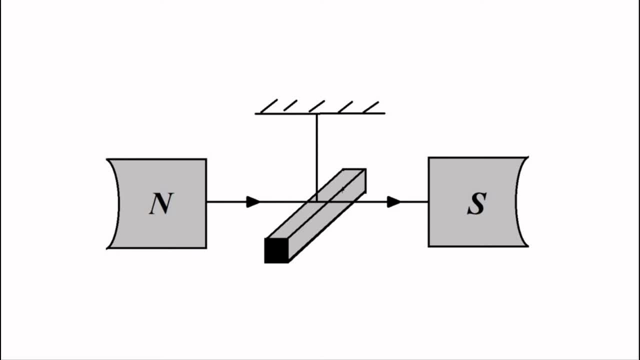 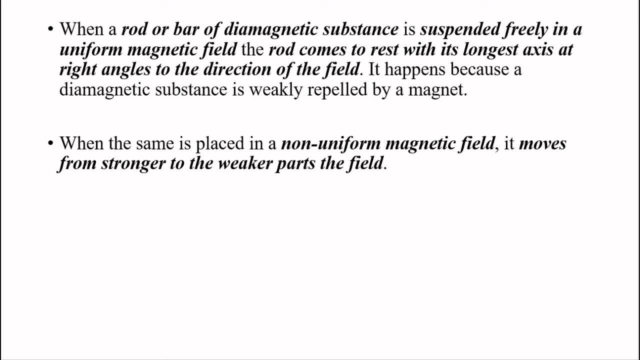 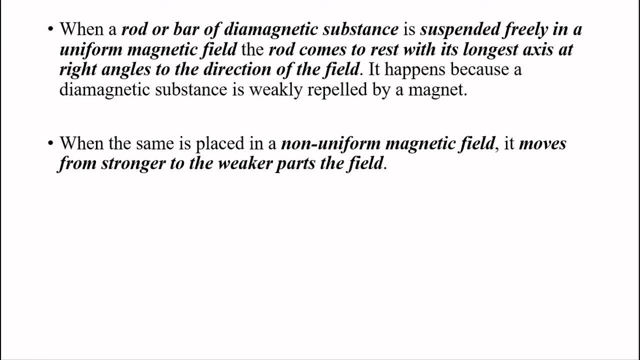 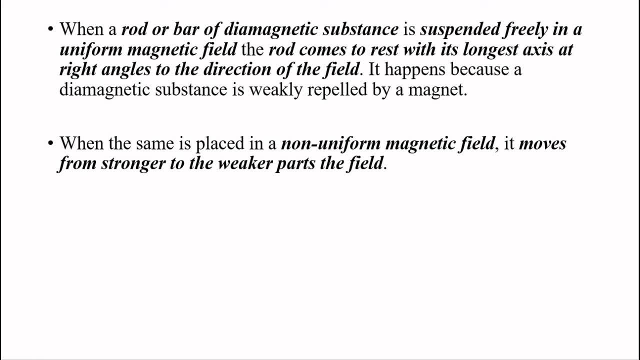 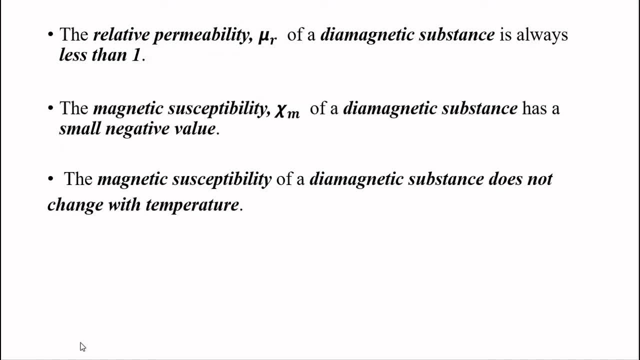 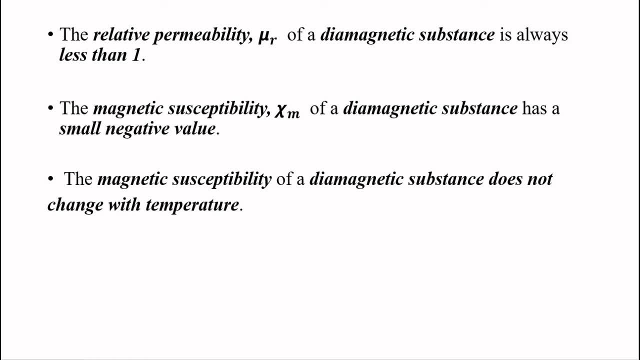 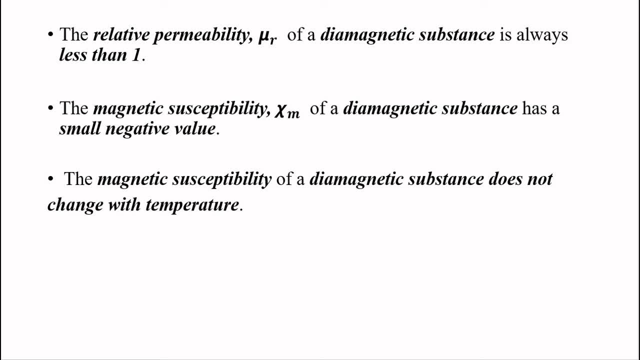 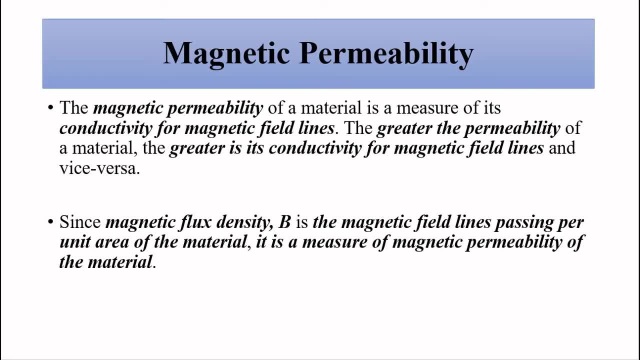 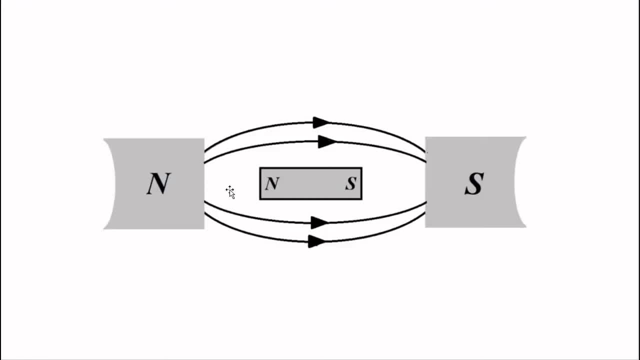 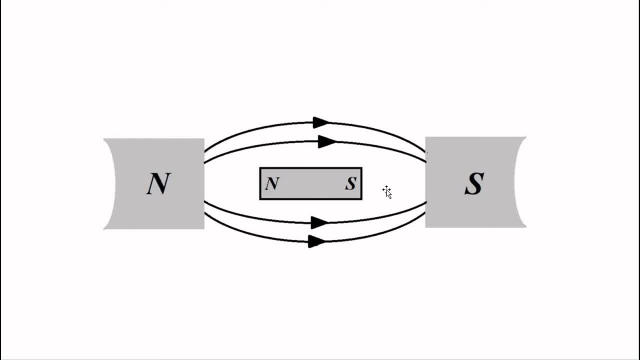 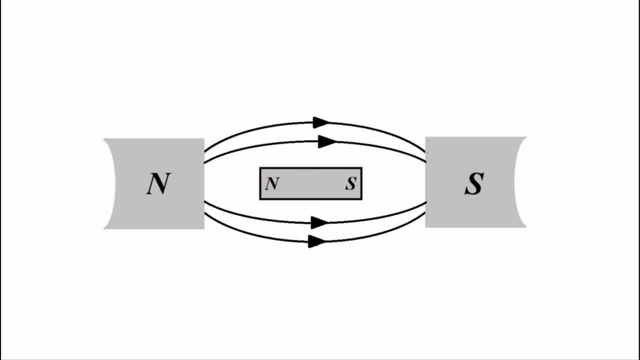 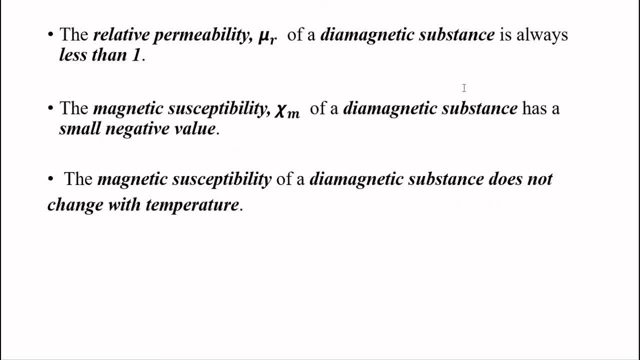 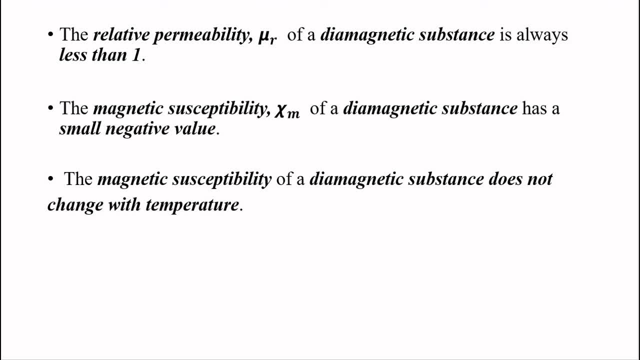 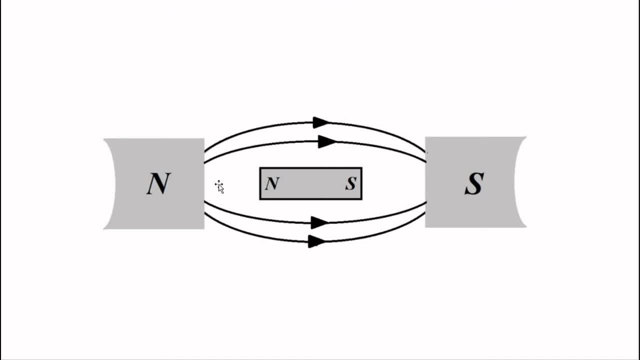 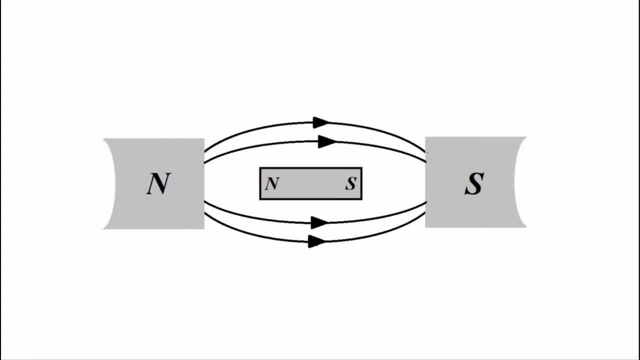 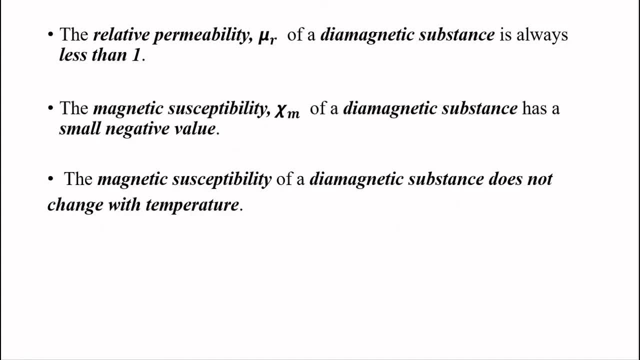 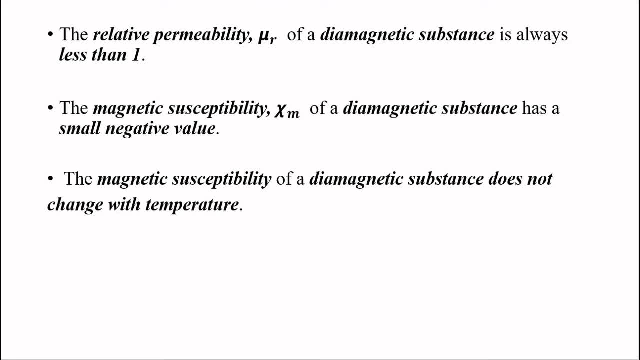 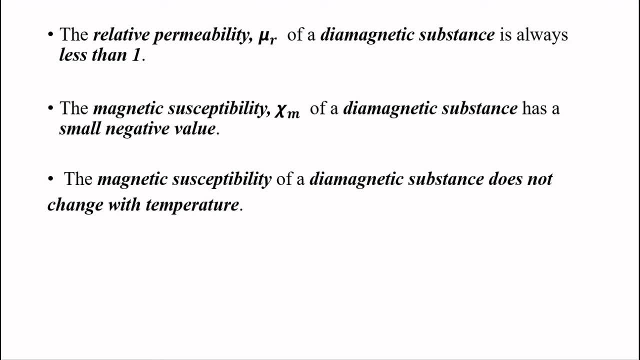 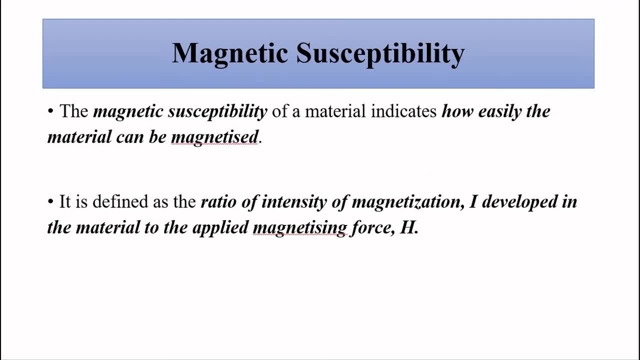 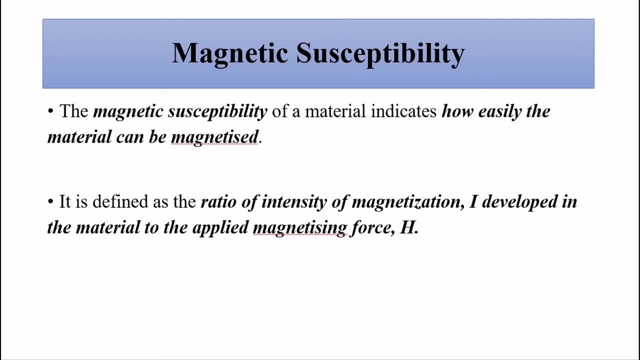 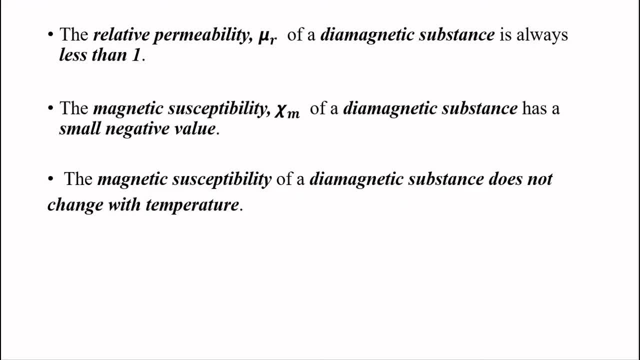 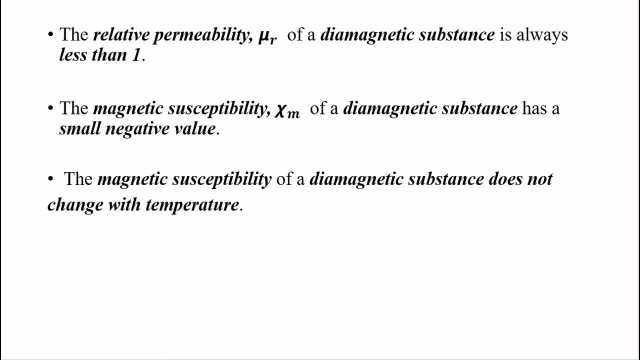 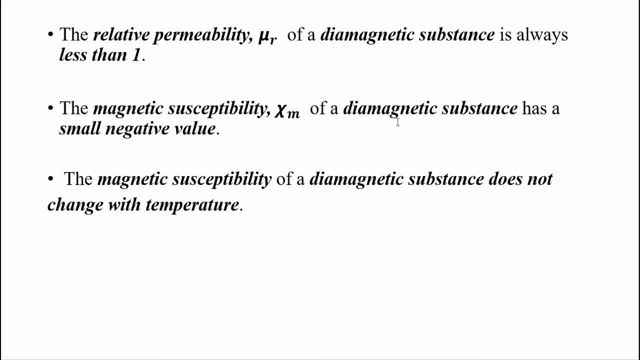 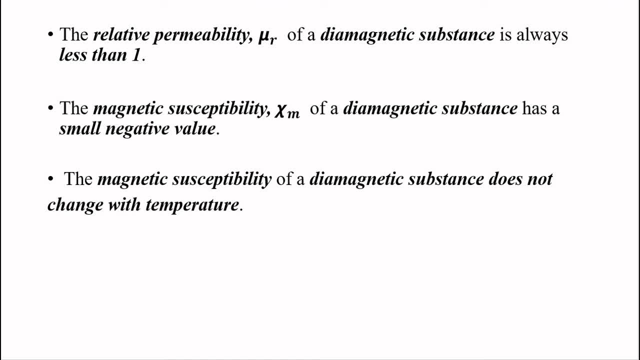 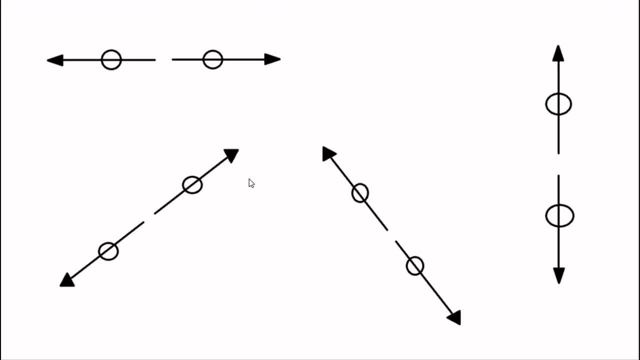 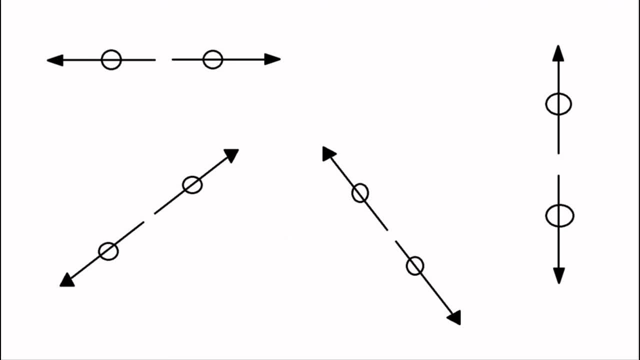 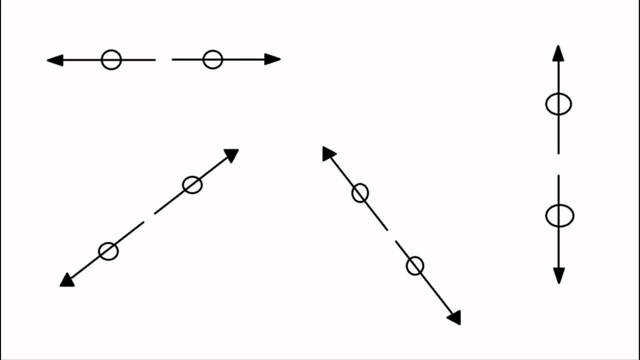 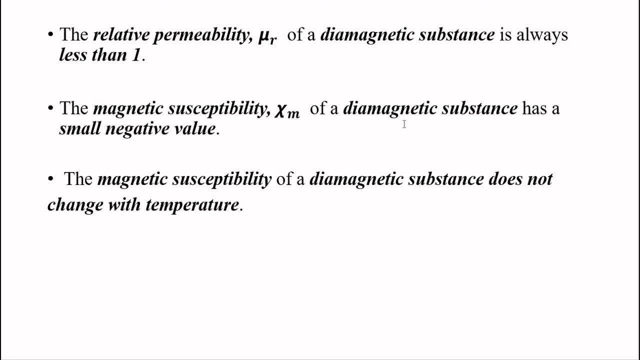 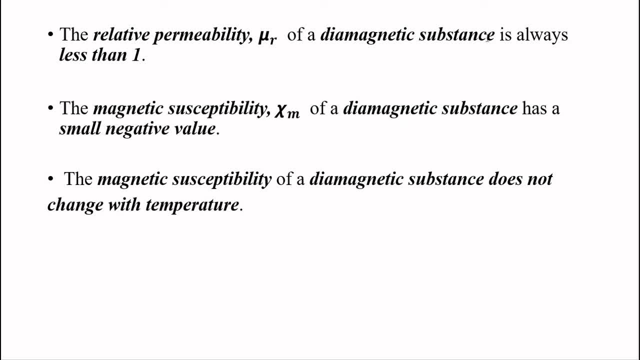 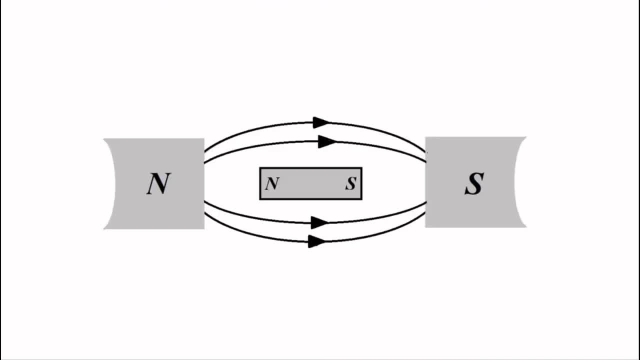 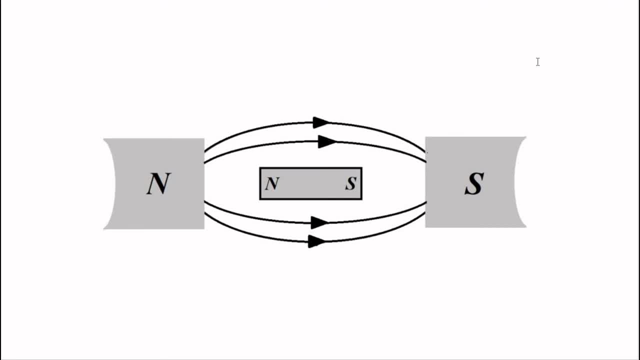 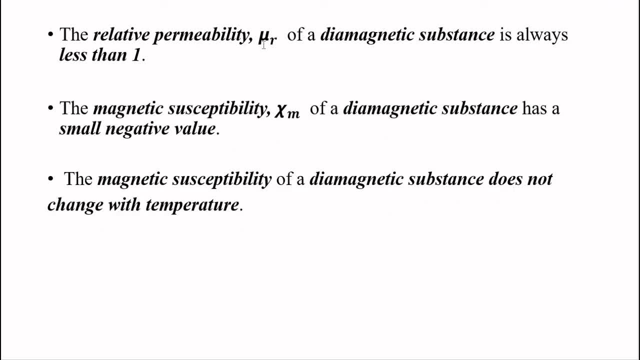 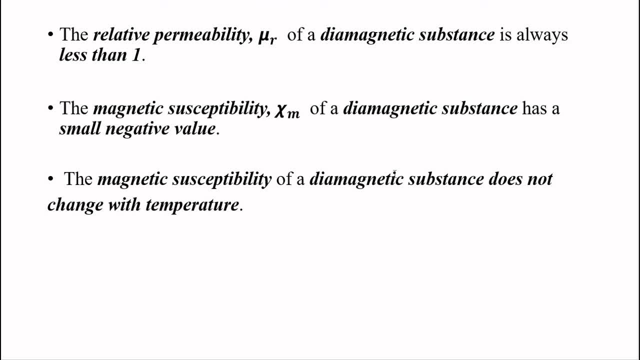 in direction, so they always cancel each other out. As you can see, with all its properties, it is a very weak form of magnetism, weak magnetic properties And also the magnetic susceptibility of diamagnetic substance. they do not change with temperature. So these are the important concepts related to first, the magnetic materials, based on how, 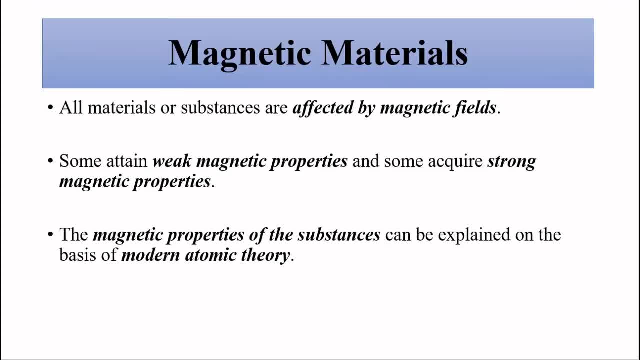 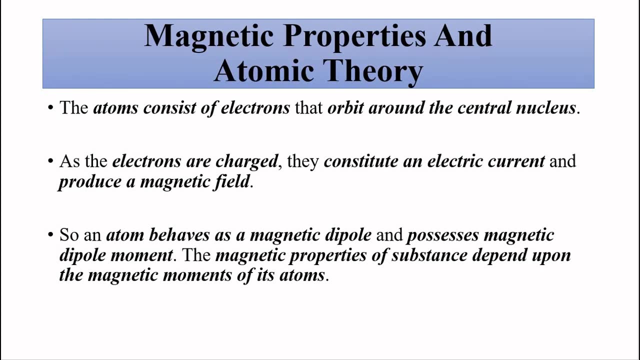 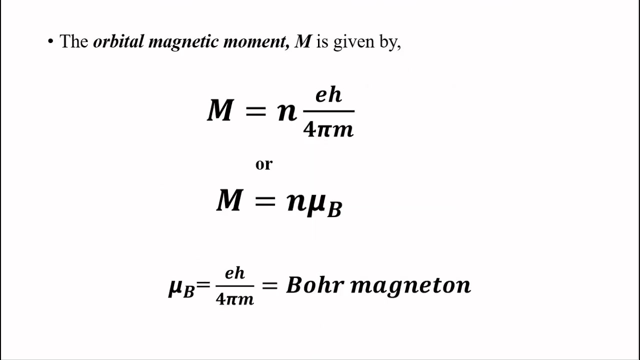 different materials. they acquire magnetic properties. why some materials attain weak form of magnetism, some strong form of magnetism? It is because of their orbital magnetic dipole movements, because of the movement of electrons around the nucleus and the orbital magnetic movement. Then the classification of magnetic materials. first we have discussed diamagnetic materials. 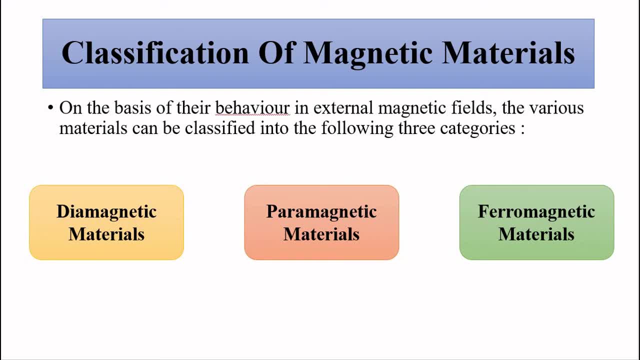 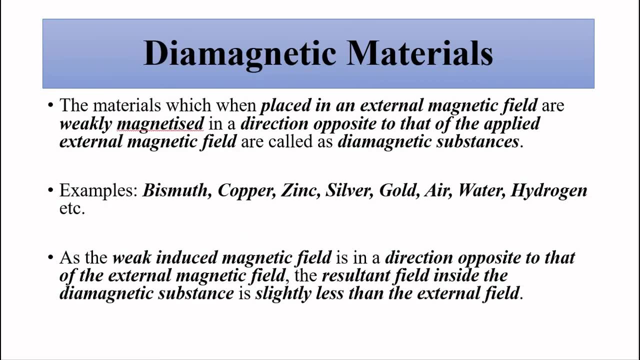 Next we will be discussing paramagnetic, Then ferromagnetic in separate videos. Diamagnetic materials: very weak form of magnetism and the magnetism it is, you know. it happens for a very small period of time in the presence of external magnetic field and as soon as.